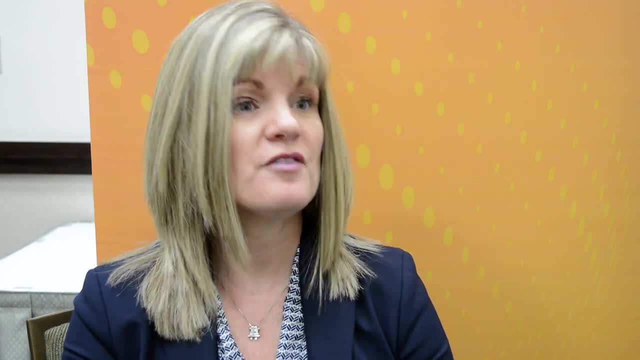 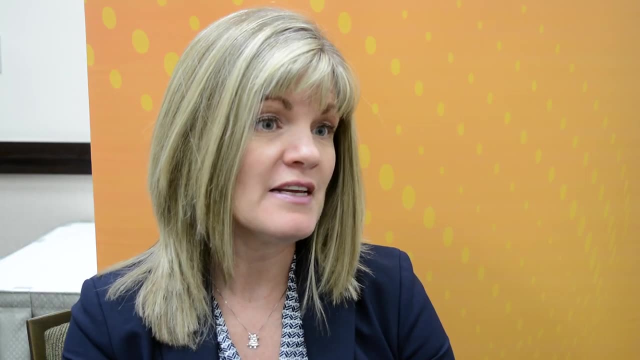 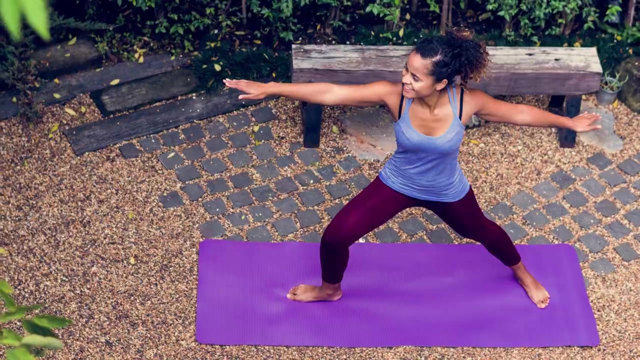 So there's a lot of musculoskeletal risk associated with prolonged sitting, The information out there that there's increased obesity, increased heart disease, all of that type of information- But what we're finding is actually, if people exercise- and they do 60 to 90 minutes of exercise a day, then their risks of prolonged sitting really are not as bad as we think. 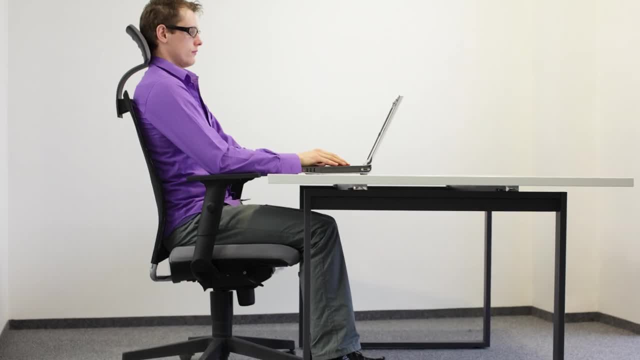 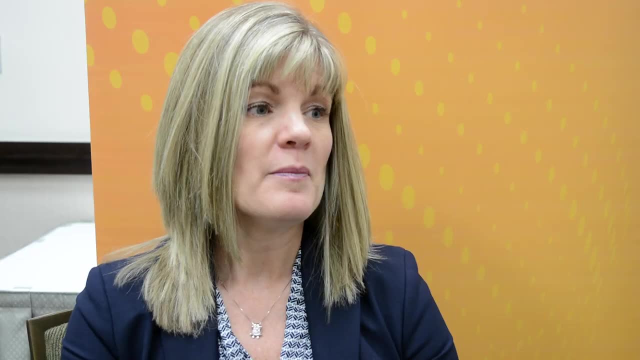 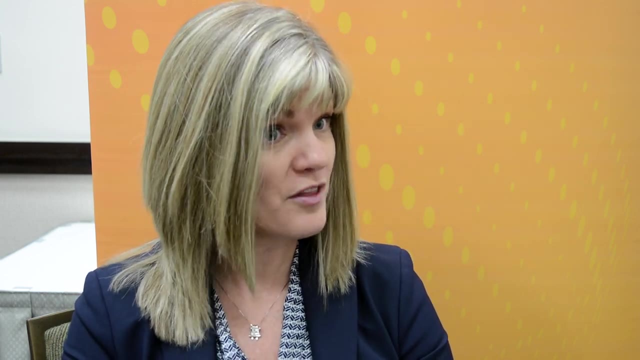 And if they're sitting in a good ergonomic chair and they're properly adjusted in their chair and they're taking the time to get up and take breaks away from their seated workstation, their risk goes way down. Now, as far as standing goes, there have been some links to increased cardiovascular risk and disease with prolonged standing. 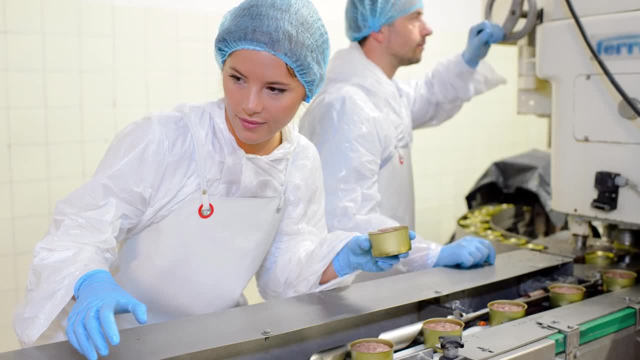 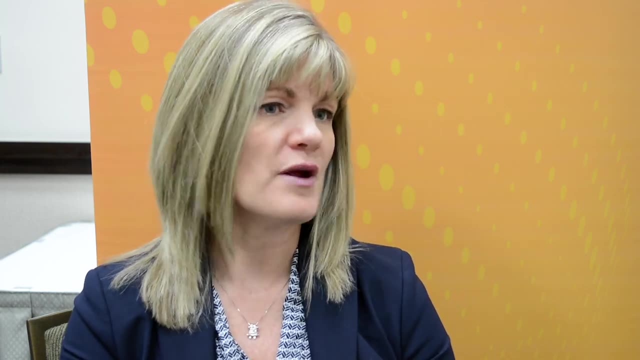 So when I say prolonged standing, I typically mean greater than six to eight hours a day. Prolonged sitting- we tend to define it as greater than six hours a day, And that's where we want to start to try to incorporate movement into our workday. 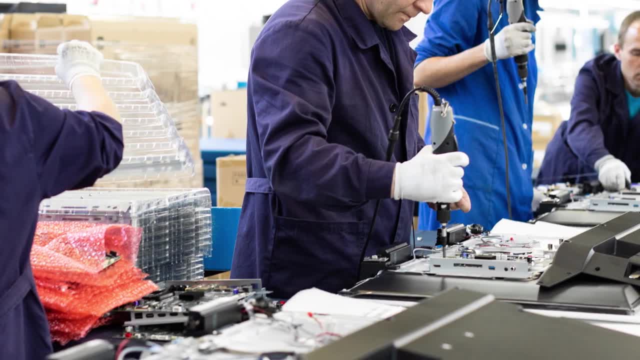 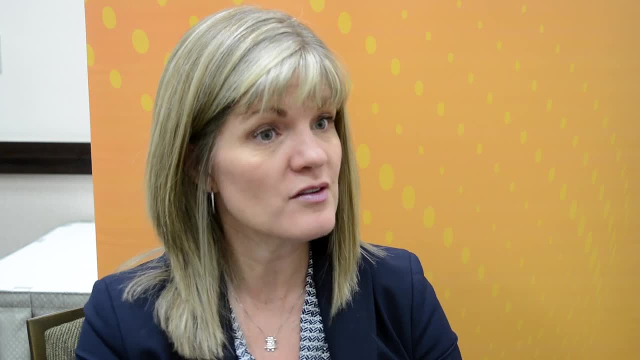 It's the static standing that's the concern in most cases. So static standing means that they're not moving, they're standing in one spot. So, again, the best thing they can do is to try to create some movement. Try to, you know, alternate legs on a footrest or take some steps. 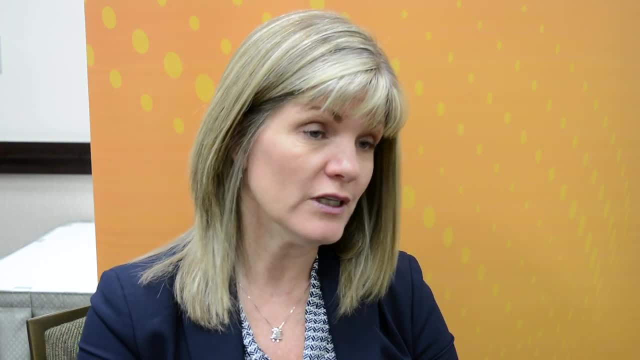 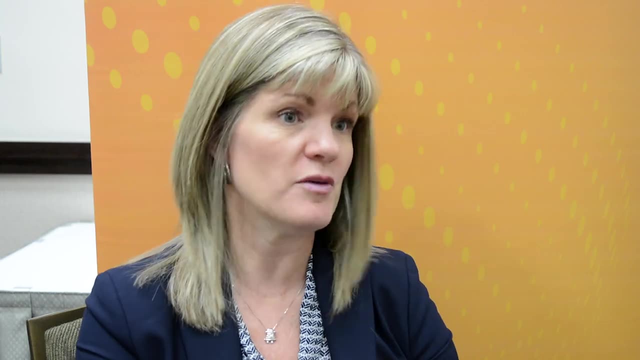 Make sure they have proper footwear. What you're wearing on your feet really will impact how you feel when you stand. Having good supportive insoles in your shoes if you're working in a manufacturing facility. put them in your safety boots If you're standing in an office environment. 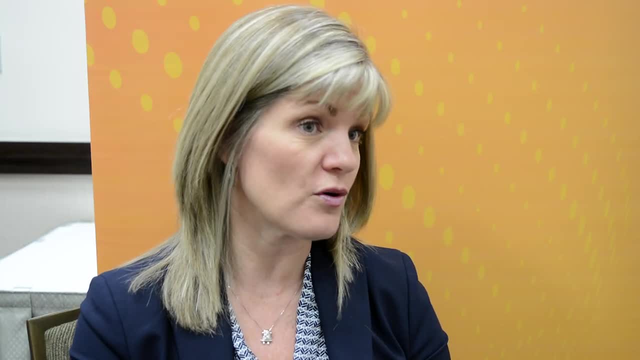 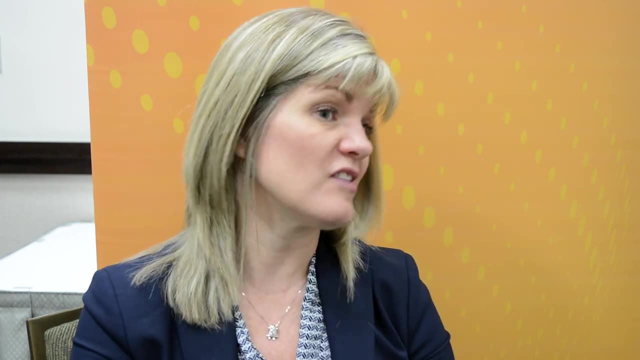 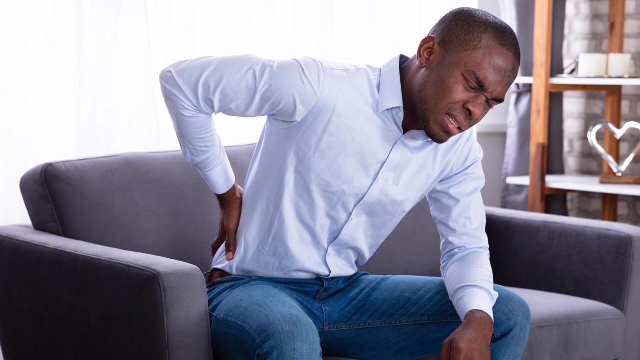 at a sit-stand station, make sure you don't have heels on, Make sure you're wearing supportive shoes. So those are the keys. The other keys are that the rest of the ergonomics of their workstation is set up properly, Because if they're standing and they're bent over now, their increased risk of sore back or other risk factors come into play. 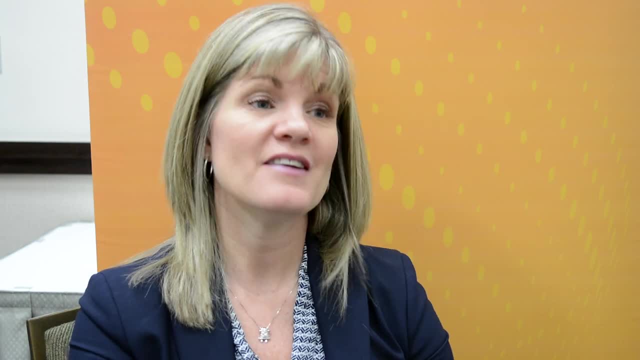 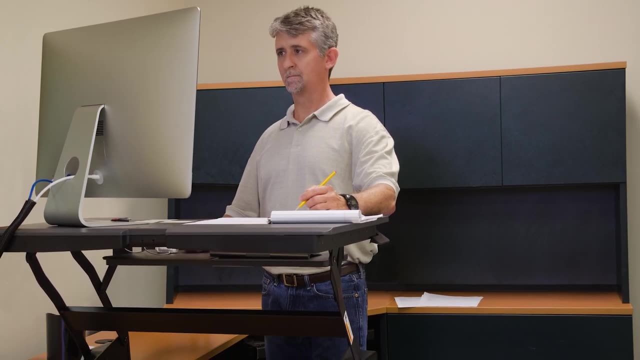 A lot of the times. people have already bought a sit-stand station and it doesn't fit them properly. They can't get their keyboard to elbow height. They can't get their monitor to eye height. The station doesn't go high enough or low enough for them. 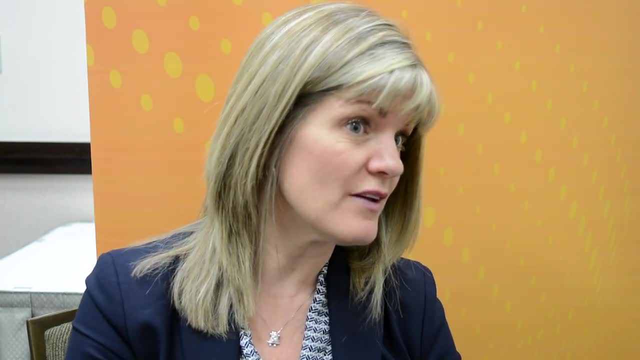 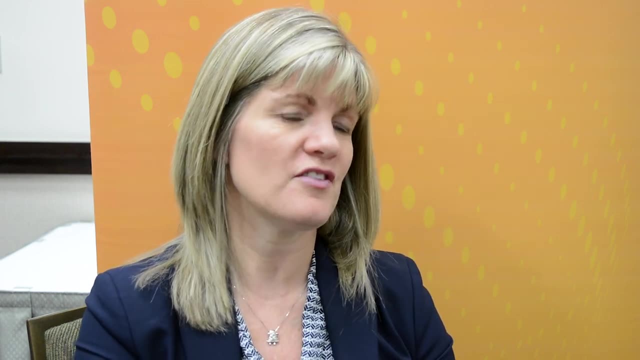 Now we're bringing in new risk factors to the workplace. We're bringing in more awkward posture. So the key here really is to implement properly and make sure that the equipment and the sit-stand station or whatever it may be that they're purchasing, will fit the person and accommodate that individual. 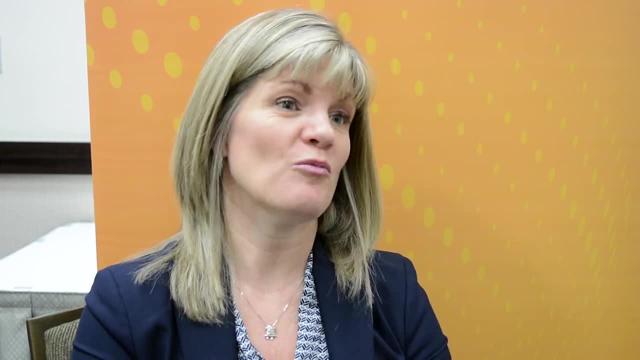 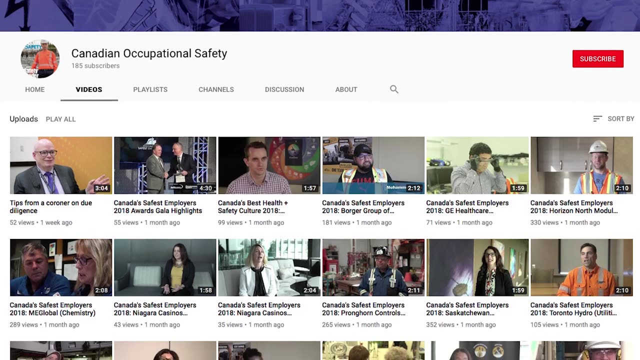 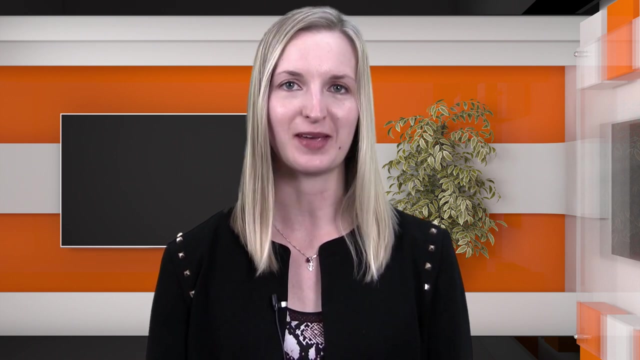 Because not one product fits everybody, And I think that's what ergonomics is all about. For more health and safety videos, subscribe to our Canadian Occupational Safety YouTube channel And don't forget to follow us on Twitter at COSMagazine For Canadian Occupational Safety. I'm Amanda Silvaker. 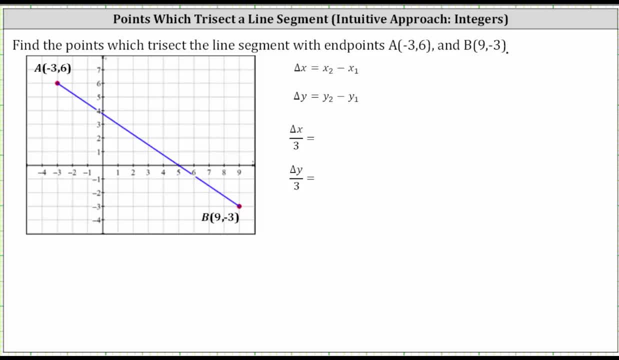 We're asked to find the points that trisect the line segment within points negative three comma six and nine comma negative three. Notice how I've already sketched the line segment on the coordinate plane. The points that trisect a line segment would be the points on the line segment. 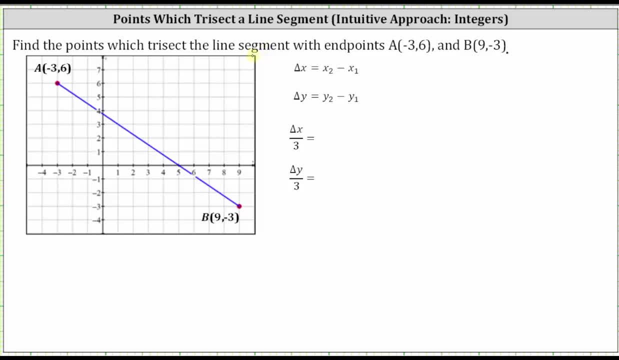 where if we cut the line segment at those points, it would create three shorter line segments, all with the same length. So for example, for segment AB, one point might be this point here Let's call it P sub one. And the second point might be, let's say here: 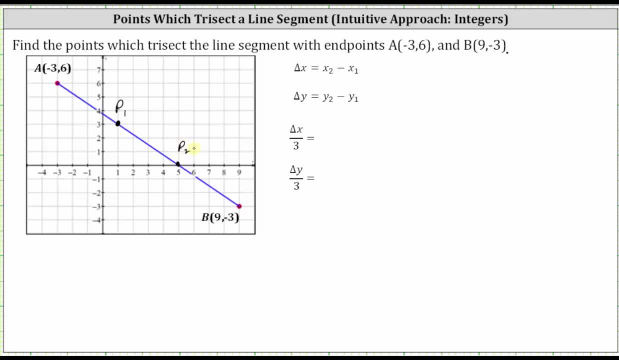 we will call the point P sub two, where if we cut the line segment at these two points it would create three line segments all with the same length. Or we can say the length of line segment AP sub one has the same length as line segment P sub one. P sub two. 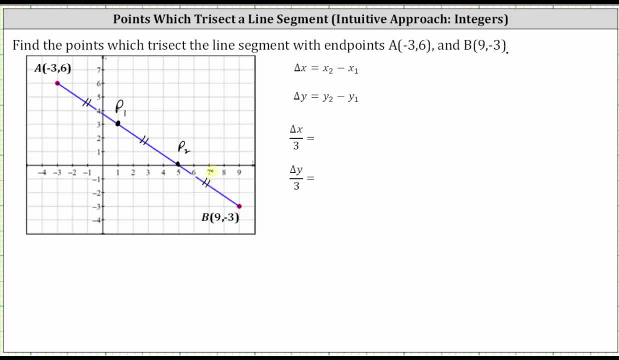 which has the same length as line segment P sub two. B. To determine the ordered pairs for P sub one and P sub two, we'll begin by determining the change of X and change of Y from point A to point B, And then we'll divide those changes by three.